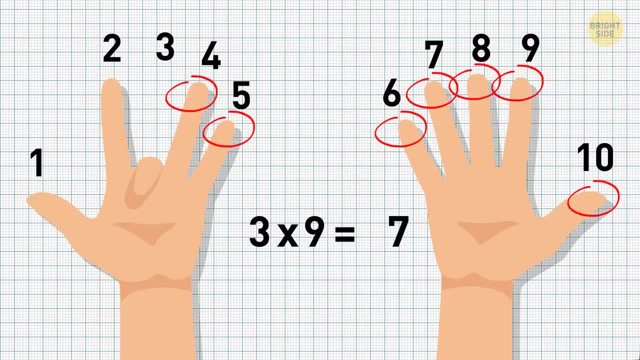 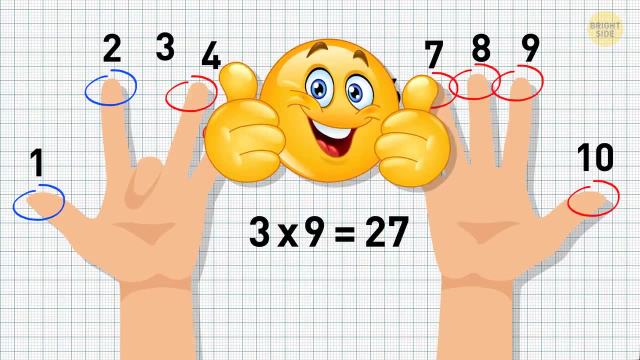 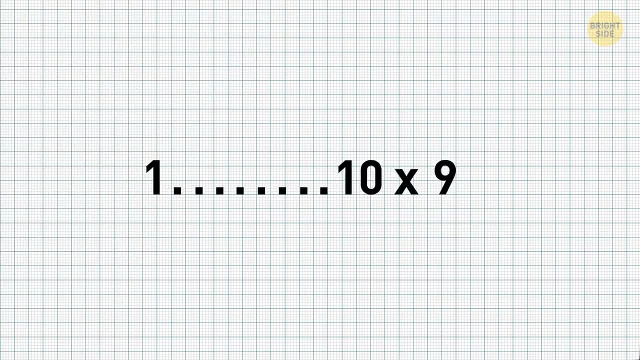 fingers. That's the first part of the answer. On the left, only two fingers are left unbent, and that's your second part. Voila, 9 times 3 equals 27.. While in the previous example we could only multiply the first 10 digits by 9,. 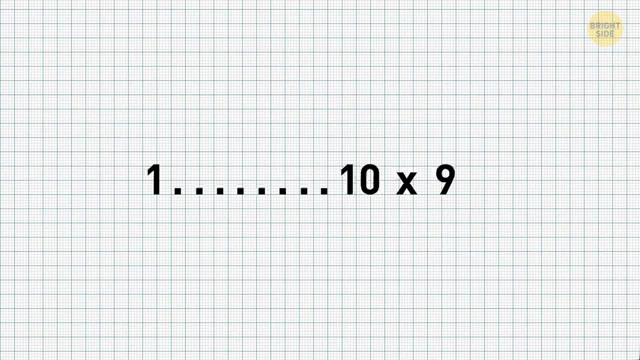 now. we'll do this trick with just about any number and it's easy as pie. Take any random large number like 1250.. Multiplying it by 9 in a conventional way without a calculator would take you some time. To make it simpler, just add a 0 at the end and 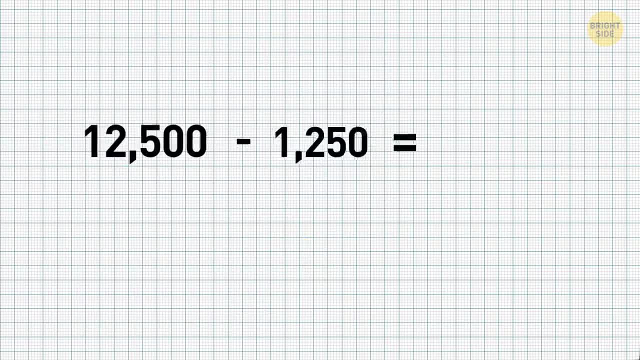 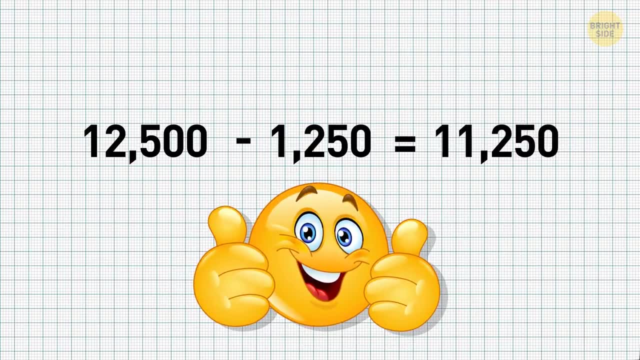 subtract from it. You can do this with any number you want, but if you don't have a calculator, just add the original number. That makes it 12,500 minus 1,250 and equals 11,250.. That's how quick it is. 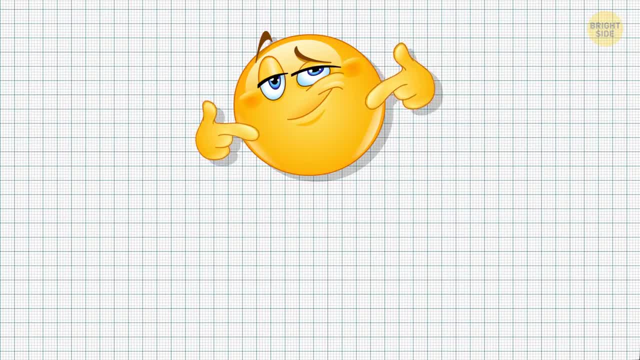 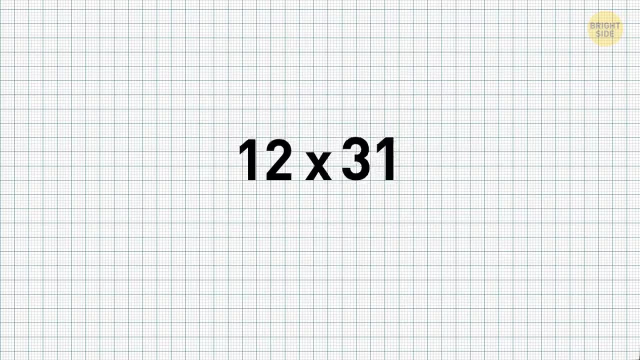 Now let's take it a step further and learn to multiply any large numbers between each other. For this we'll use a method taught in Japanese schools. Let's take 12 multiplied by 31 as an example. In this method, the numbers multiplied are represented by 10s and 1s. 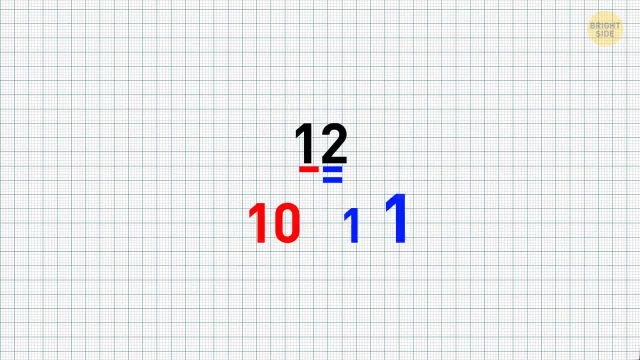 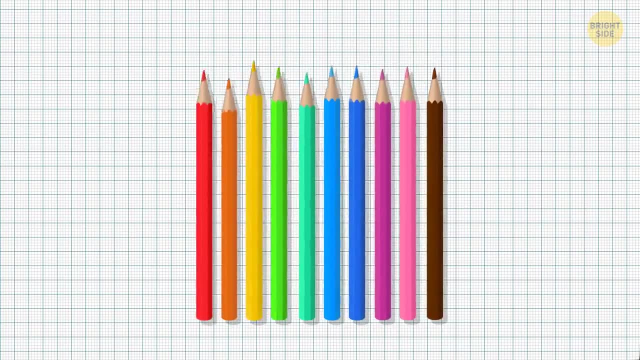 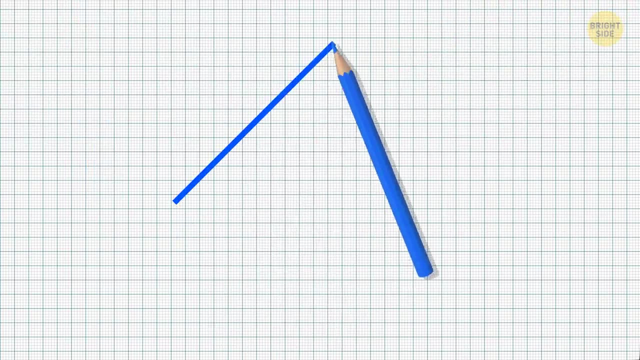 12 will be one 10 and two 1s, and 31 will be three 10s and a 1.. Now take a piece of paper and some colored pencils, ideally 4.. We'll draw the numbers, making them visual. First, draw one diagonal line left to right, going up. It will represent: 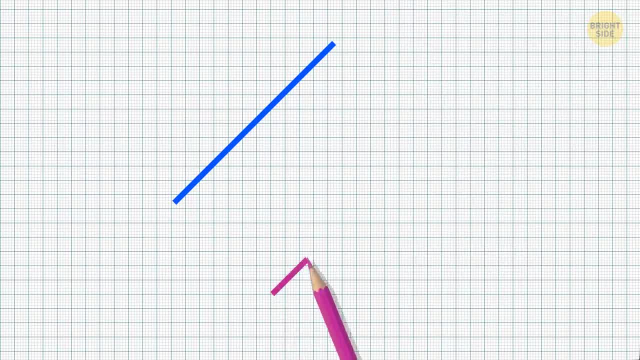 10 in 12.. Take another pencil and leave a gap below. Draw two more diagonal lines in parallel to the first one. This is our 12.. This is our 12. For number 31,. we'll draw some more diagonal lines. Only these ones will go in the opposite. 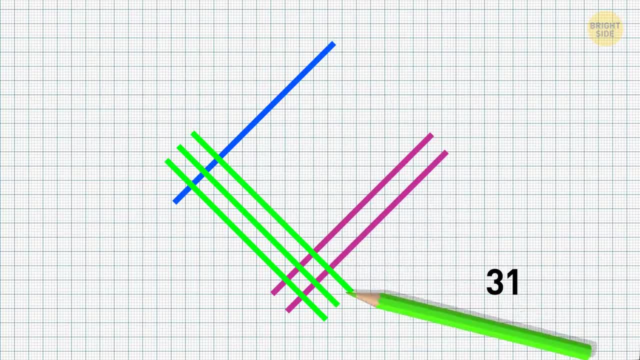 direction and cross our original lines. So it's three lines left to right going down for three 10s and one more line with a gap above the first three for a 1.. Don't forget to use differently colored pencils as well, to avoid confusion, while you're still not used to this method. 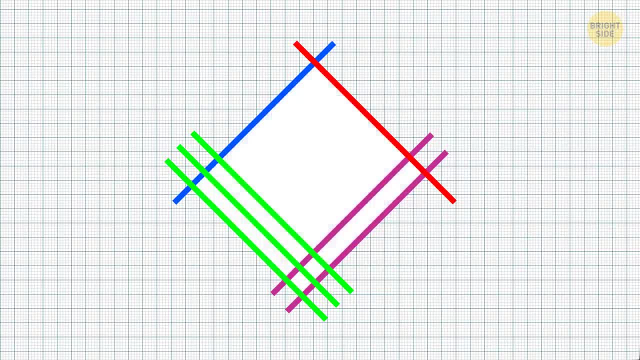 Now you have a diamond shape made of intersecting lines. To calculate the result, count the times all the lines cross each other at each corner of the diamond and write down those numbers at each intersection. You should have 3 at the left corner of the 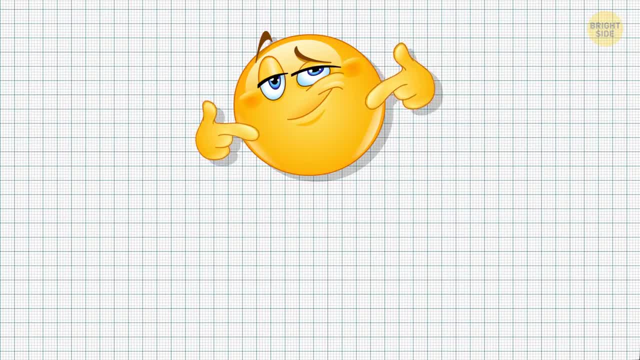 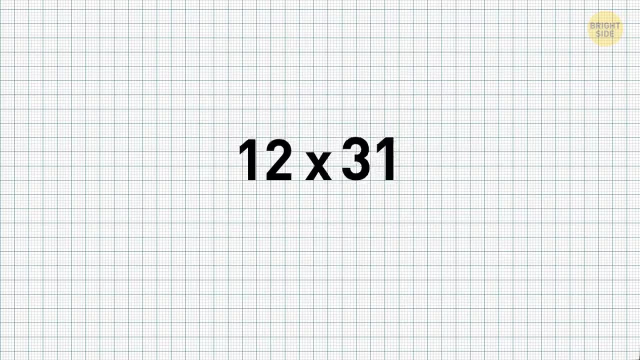 Now let's take it a step further and learn to multiply any large numbers between each other. For this we'll use a method taught in Japanese schools. Let's take 12 multiplied by 31 as an example. In this method, the numbers multiplied are represented by 10s and 1s. 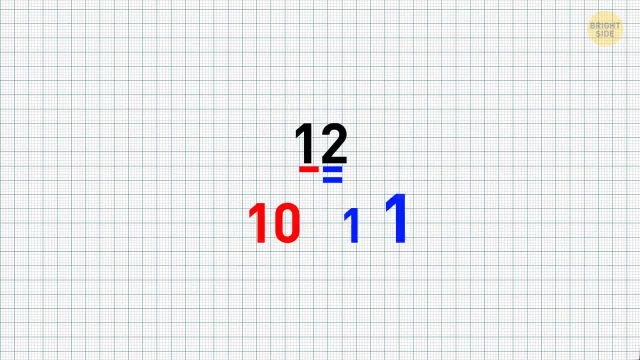 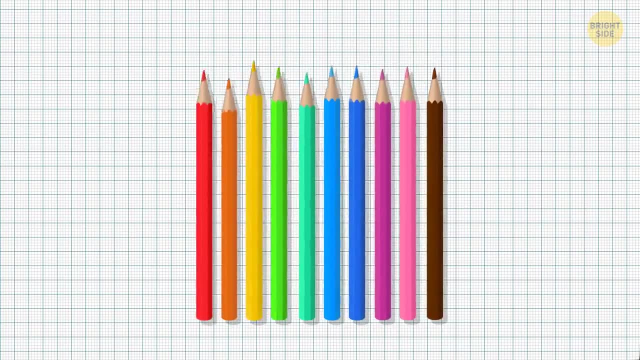 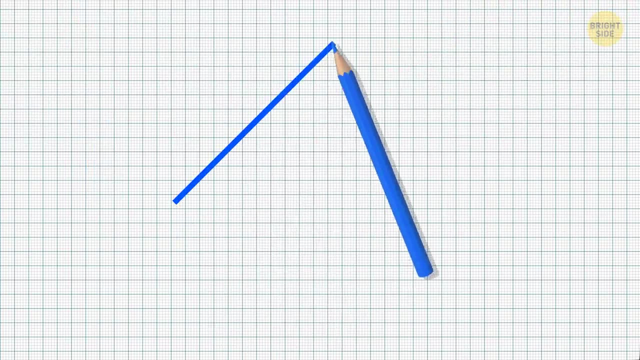 12 will be one 10 and two 1s, and 31 will be three 10s and a 1.. Now take a piece of paper and some colored pencils, ideally 4.. We'll draw the numbers, making them visual. First, draw one diagonal line left to right, going up. It will represent: 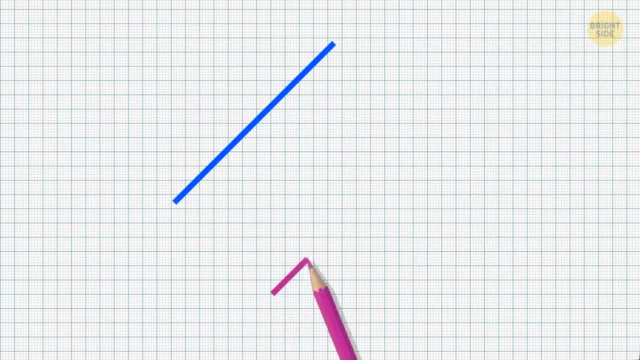 10 in 12.. Take another pencil and leave a gap below. Draw two more diagonal lines in parallel to the first one. This is our 12.. This is our 12. For number 31,. we'll draw some more diagonal lines. Only these ones will go in the opposite. 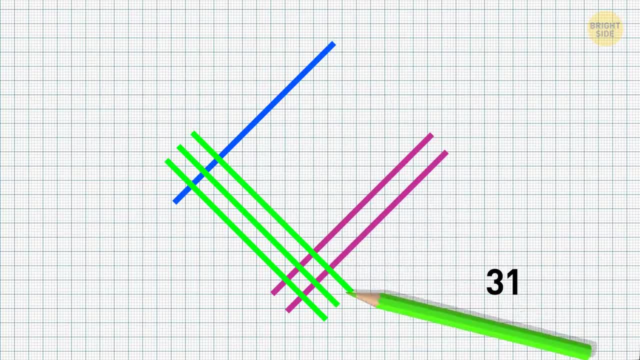 direction and cross our original lines. So it's three lines left to right going down for three 10s and one more line with a gap above the first three for a 1.. Don't forget to use differently colored pencils as well, to avoid confusion, while you're still not used to this method. 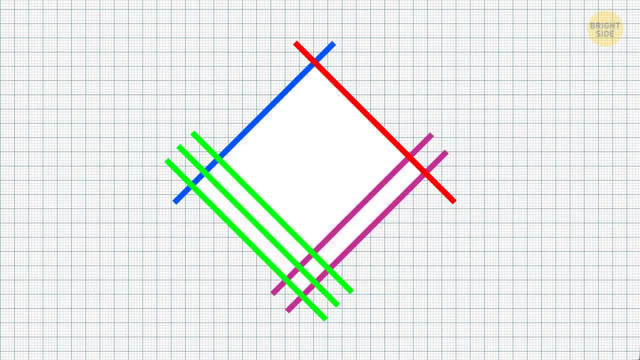 Now you have a diamond shape made of intersecting lines. To calculate the result, count the times all the lines cross each other at each corner of the diamond and write down those numbers at each intersection. You should have three at the left corner of the diamond, two at the right. 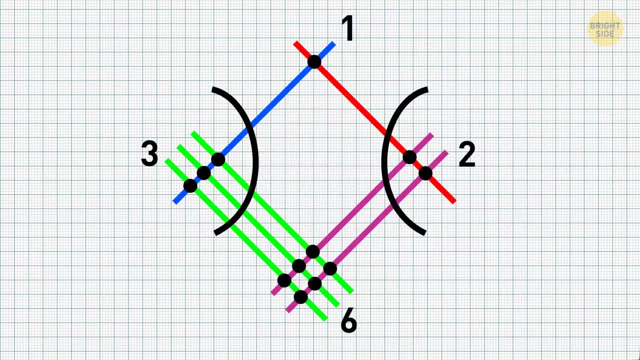 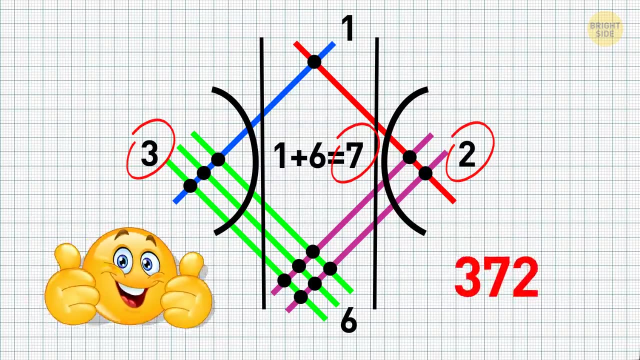 corner, one at the top and six at the bottom, Leaving the side corners alone for now. add the top and bottom values together, That'll be seven, And if you now divide the diamond shape into three parts with vertical lines, you'll get your desired result 372.. There's a trick to this. 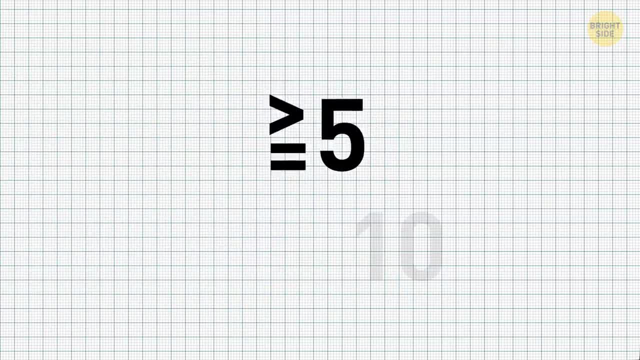 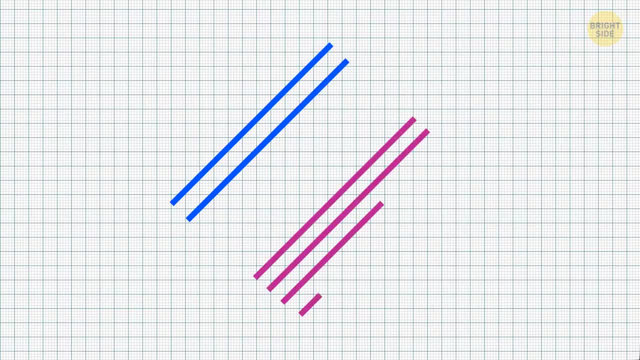 If you're trying to do it with numbers ending with five ones or more, you might get double-digit results when counting the intersections. So let's see how to deal with those, taking 25 multiplied by 37 as an example. So we draw two diagonal lines for two 10s and five more for five ones. That's 25 for us. 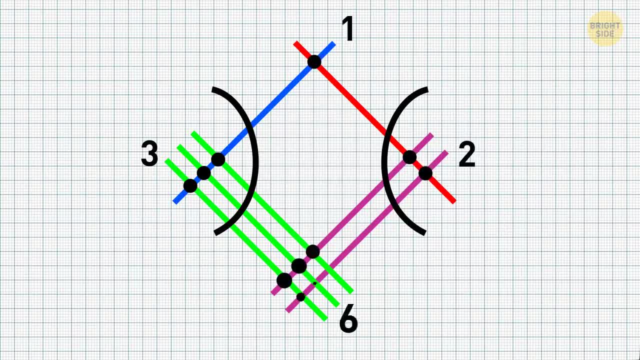 diamond: 2 at the right corner, 1 at the top and 6 at the bottom, Leaving the side corners alone for now. Add the top and bottom values together, That'll be 7.. And if you now divide the diamond shape into three parts with vertical lines, you'll get your desired result 372.. 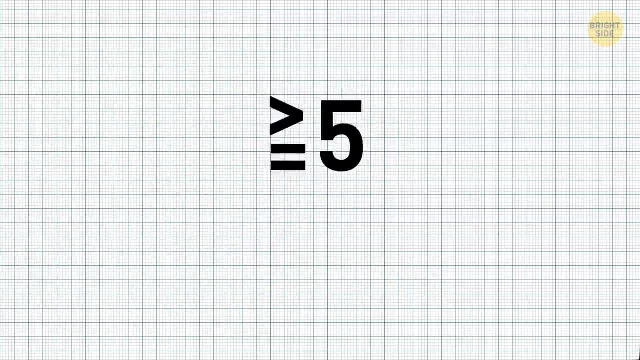 Woohoo, Catchy. catch, though, If you're trying to do it with numbers ending with five 1s or more, you might get double-digit results when counting the intersections. So let's see how to deal with those taking 25 multiplied by 37 as an example. 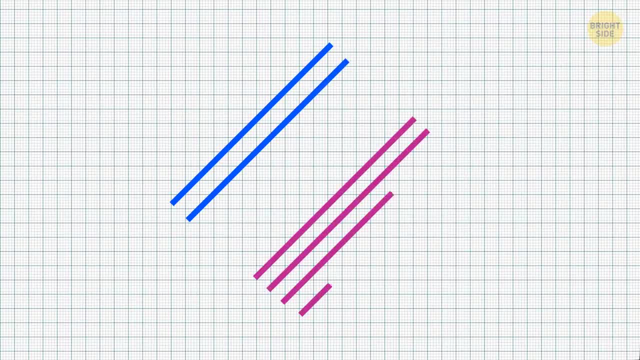 So we draw two diagonal lines for two 10s and five more for five 1s. That's 25 for us. Now there are three crossing lines for three 10s and seven more for seven 1s, And there's our 37.. 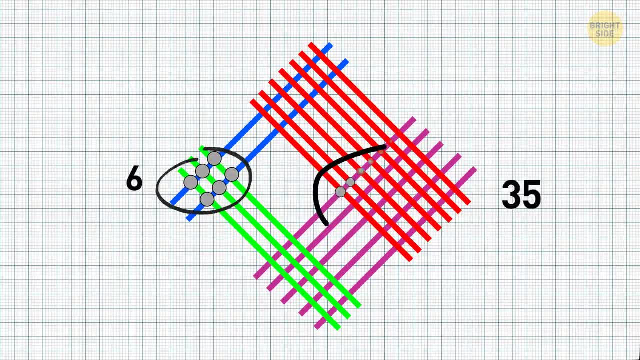 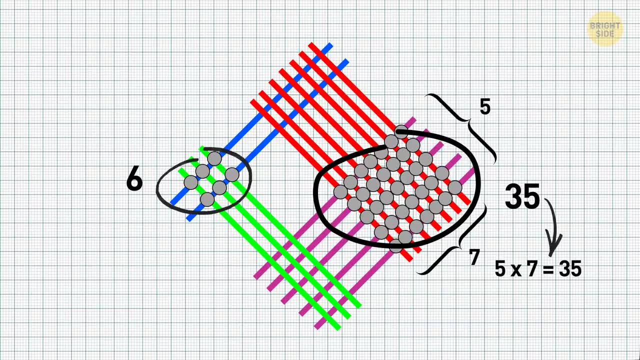 Now we count the dots: 6 at the left corner of the diamond, 35 at the right corner. The times table will help you out a lot here. to make it quick, Just multiply 5 by 7.. 14 at the top. 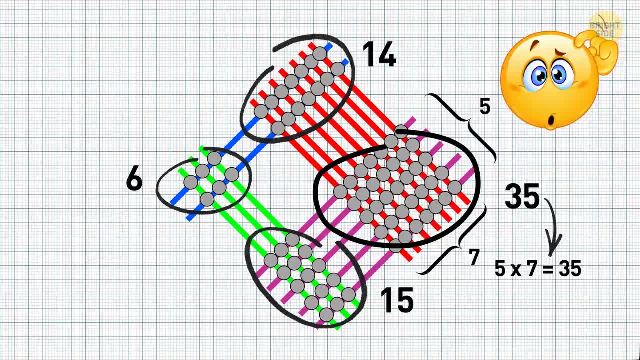 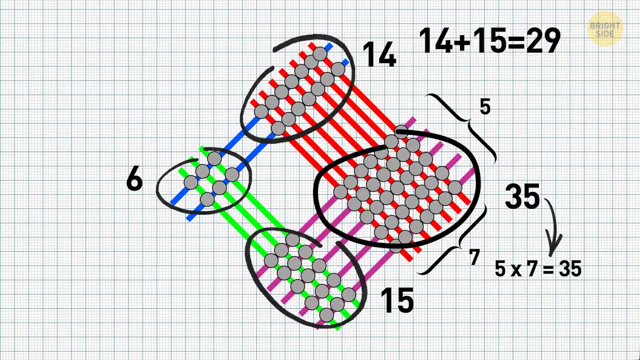 and 15 at the bottom. A lot of double-digit numbers here. First let's add the top and bottom results, as we did last time. 14 plus 15 equals 29.. Now we have 6,, 29, and 35.. Take the right-most. number and only leave the 5 in it. Now we have 6,, 29, and 35.. Take the right-most number and only leave the 5 in it. Now we have 6,, 29, and 35.. Take the right-most number and only leave the 5 in it. 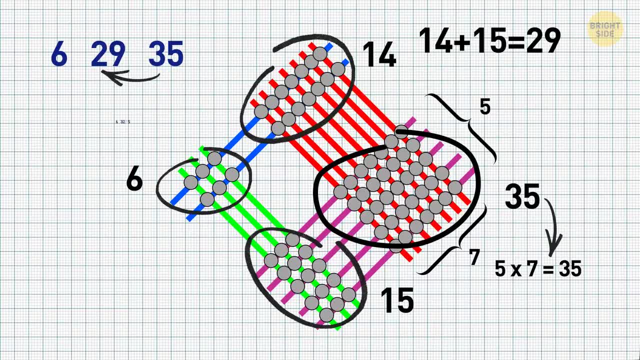 Transferring the 3 to the middle number and adding it to the sum, You'll get 6,, 32, and 5.. Do the same with 32 now. Only leave the 2 and transfer the 3 to the left. 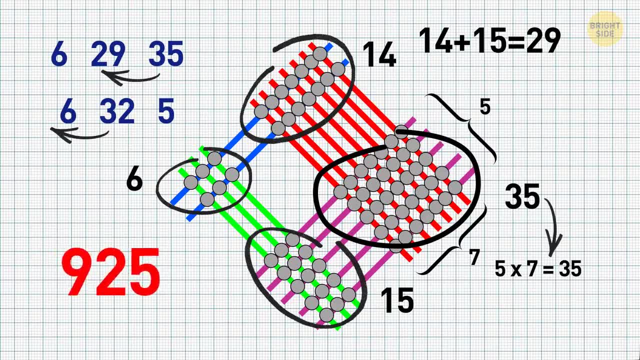 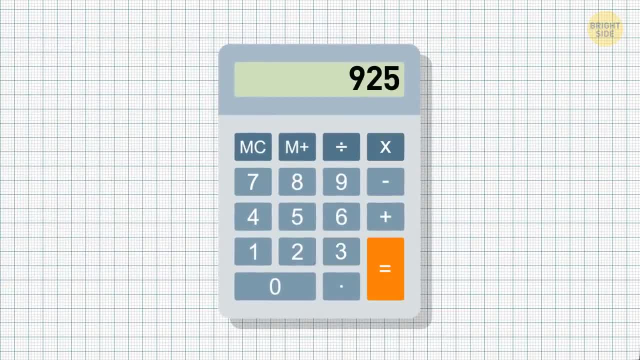 Add it to the 6 and voila, You've got your answer. Check yourself with a calculator if you want, but 925 really is the correct result. And finally, the same method can be applied to even larger three-digit numbers. Let's take 322,. 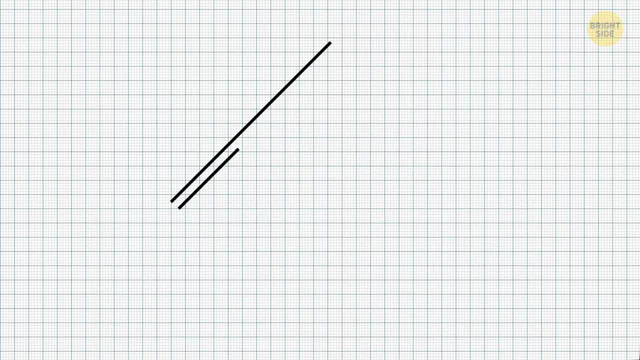 and add it to the sum. Now you'll get 322, and 432.. Let's see how it goes. The numbers that we draw first we'll add by 14, as an example. First we draw 322, just as we did previously. Only now the hundreds are a separate set of. 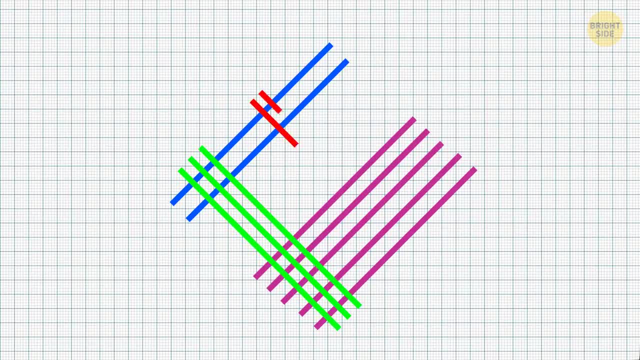 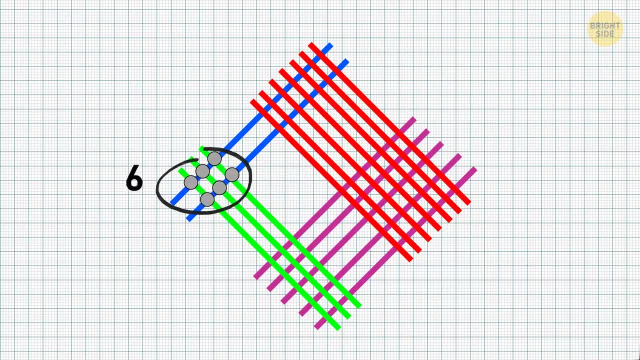 Now there are three crossing lines for three 10s and seven more for seven ones, And there's our 37. We count the dots: six at the left corner of the diamond, 35 at the right corner. The times table will help you out a lot here. to make it quick, Just multiply five by seven. 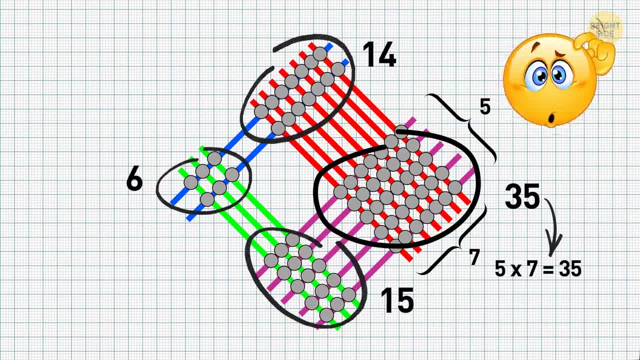 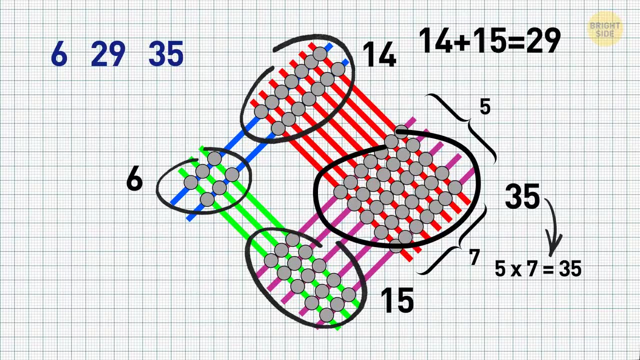 14 at the top and 15 at the bottom. A lot of double-digit numbers here. First, let's add the top and bottom results, as we did last time. 14 plus 15 equals 29.. Now we have six, 29, and 35. Take the rightmost number and only leave the five in it. 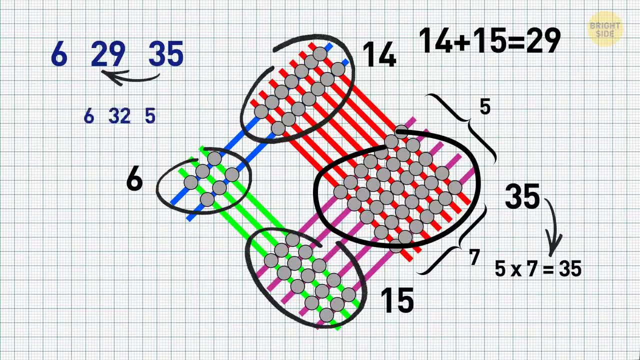 Transferring the three to the middle number and adding it to the sum, You'll get six, 32, and five. Do the same with 32. now Only leave the two and transfer the three to the left. Add it to the six and voila, You've got your answer. 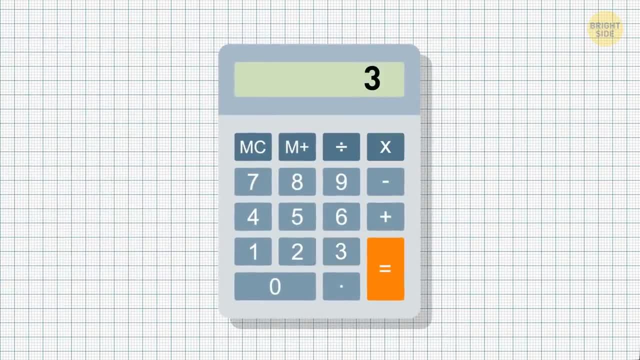 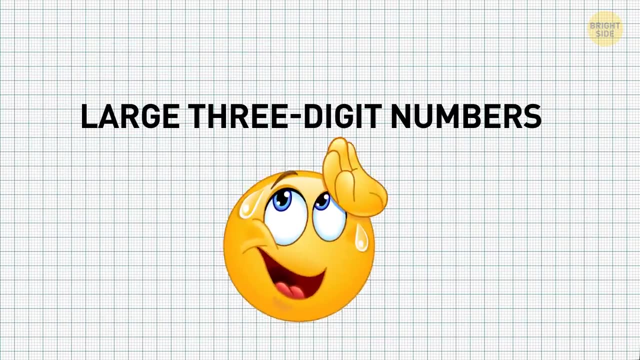 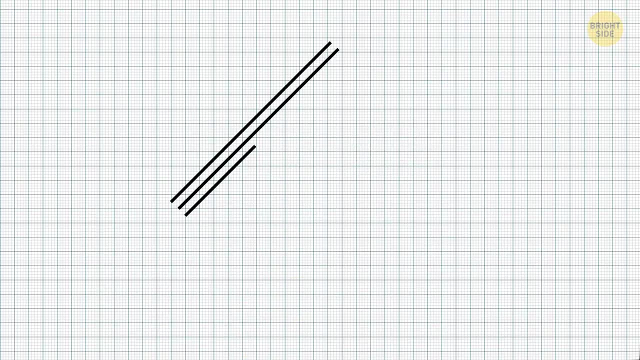 Check yourself with the calculator if you want, but 925 really is the correct result. And finally, the same method can be applied to even larger three-digit numbers. Let's take 322, multiply by 7, by 14 as an example. First we draw 322, just as we did previously. Only now the 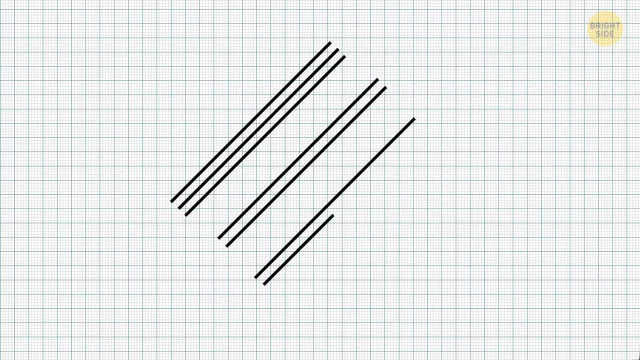 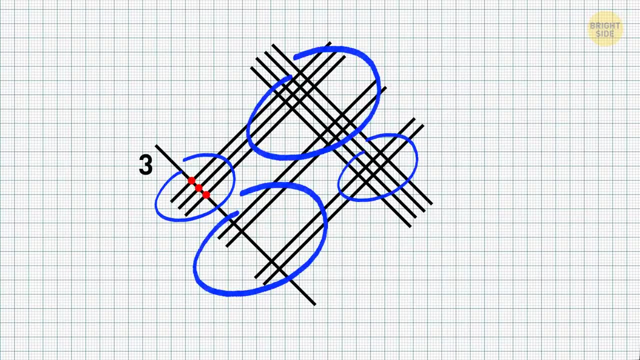 hundreds are a separate set of diagonal lines. There will be 3,, 2 and another 2.. Next add the crossing lines of 14,, 1 and 4.. You can see now we have not 3 but 4 sections. so let's count the dots. That's 3 in the leftmost section, 12 at the 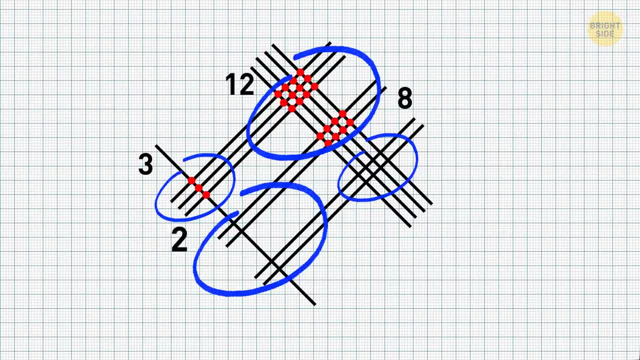 first top, 8 at the second top 2 and 2 at the first and second bottom intersections and 8 in the rightmost section. Adding the first top and bottom dots we get 14, and adding the second ones, we get 10, and the result is 3, 14, 10. 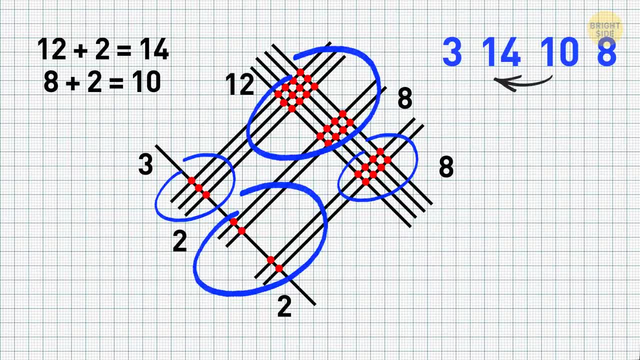 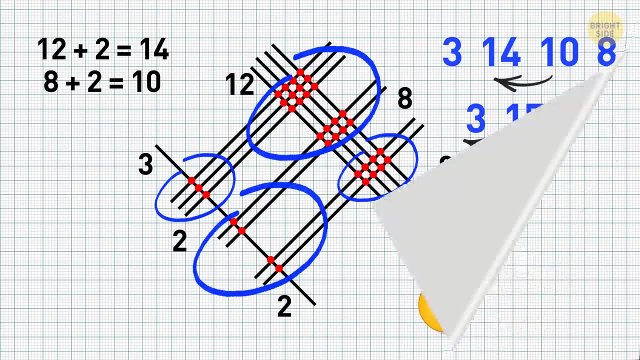 and 8.. And now you already know what to do: Transfer the 1 from 10 left, add it to 14, then transfer the 1 from the resulting 15 left too, And here you go: 4508 is your answer, The multiplication. 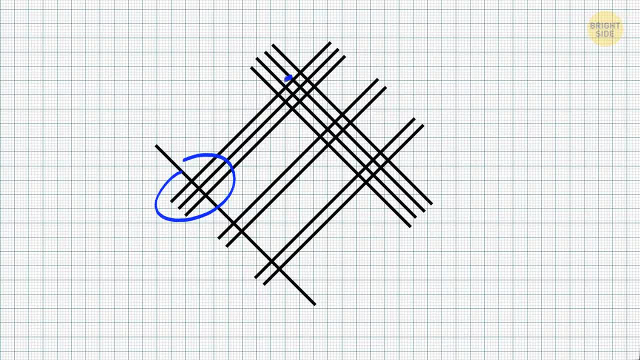 diagonal lines. There will be 3,, 2, and another 2.. Next add the crossing lines of 14,, 1, and 4.. You can see now we have not 3, but 4 sections. So let's count the dots. 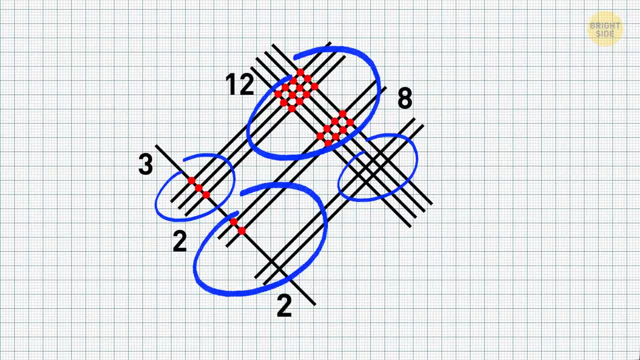 8 at the second top, 2 and 2 at the first and second bottom intersections and 8 in the rightmost section. Adding the first top and bottom dots, we get 14, and adding the second ones, we get 10.. 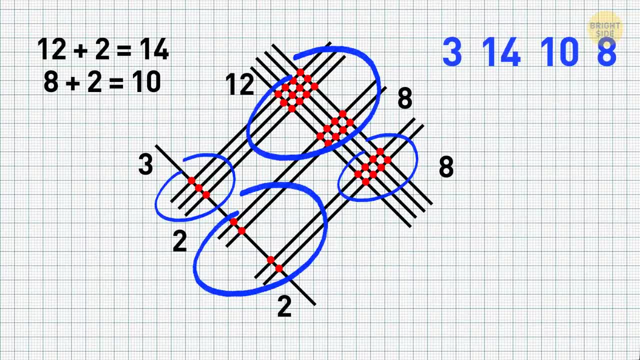 And the result is 3,, 14,, 10, and 8.. And now you already know what to do: Transfer the 1 from 10 left, Add it to 14.. Then transfer the 1 from the resulting 15 left too. 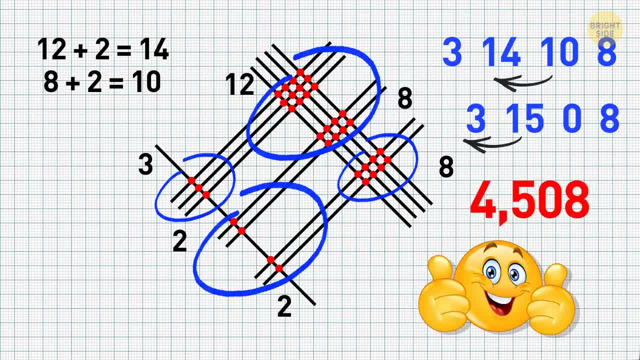 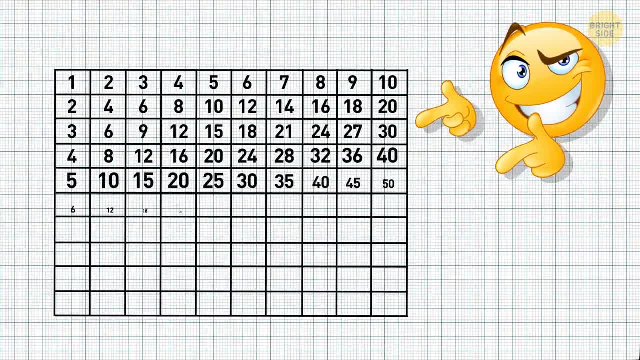 And here you go. 4,508 is your answer. The multiplication table ends with 10, and most people end up memorizing it sooner or later. But there's also a way to take it a step further and learn to multiply by 11 just as quickly. 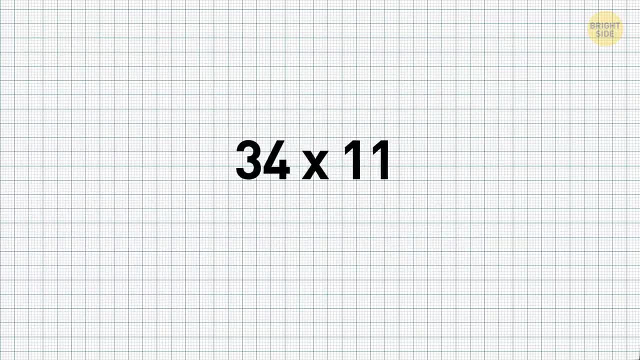 Let's take 34 as an example and multiply it by 11.. First, separate the digits making it 3. And 4, with a space between them. In that space, put the sum of these two digits, 3 plus 4, equals 7.. 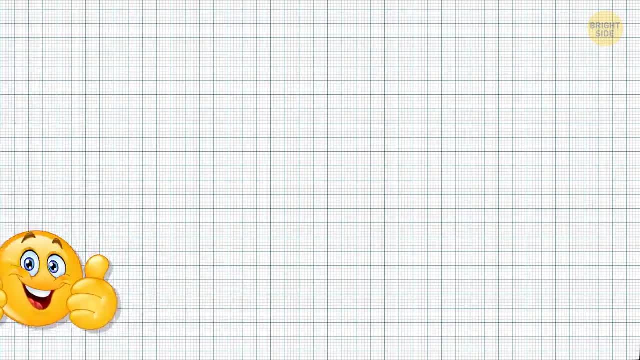 That's your answer: 374.. With some numbers, addition may result in a two-digit number. That's the case with, say, 87.. You'll get 8,, 15, and 7.. To get your actual result, add the first digit and the tens place of the sum. 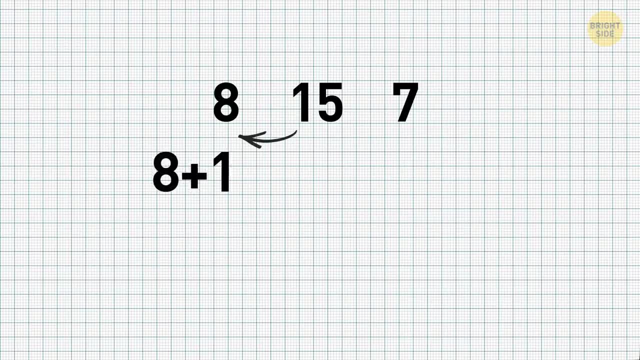 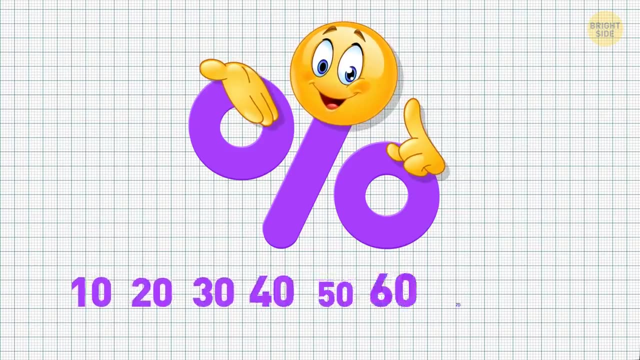 Leaving the ones alone, That will be 8.. Plus Plus 1. 5 and 7,, which results in 957.. If you know the multiplication table well enough, finding out percentages will be a piece of cake. The only downside of the following method is that it can only be used with round percentages of round numbers. 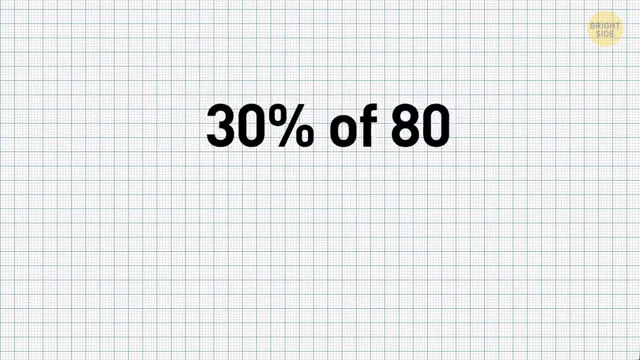 But hey, that's already something. So if you want to find out 30% of 80, you just need to ditch the zeros and multiply the tens places of these two numbers 3. Multiplied by 8 will be 24.. 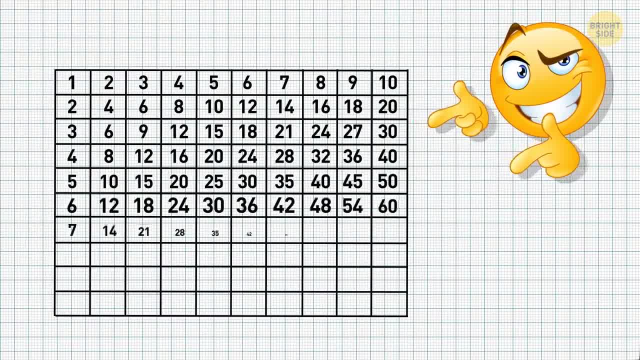 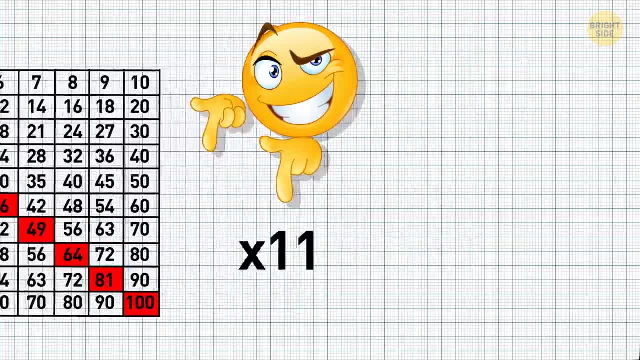 table ends with 10 and most people end up memorizing it sooner or later. But there's also a way to take it a step further and learn to multiply by 11 just as quickly. Let's take 34 as an example and multiply it by 11.. First, separate the. 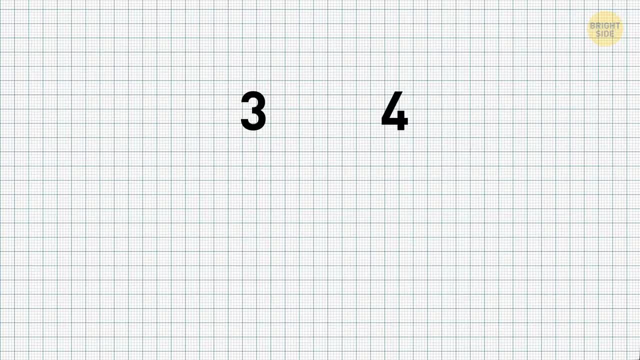 digits, making it 3 and 4, with a space between them. In that space, put the sum of these two digits, 3 plus 4, equals 7.. That's your answer: 374.. With some numbers, addition may result in a two-digit number, That's. 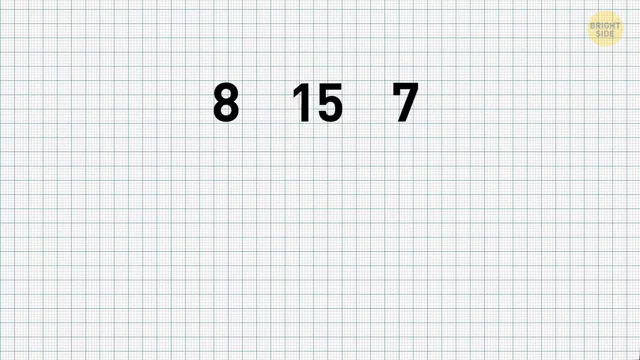 the case with, say, 87. You'll get 8,, 15 and 7.. To get your actual result, add the first digit and the tens place of the sum. leaving the ones alone, That will be 8 plus 1,, 5 and 7.. 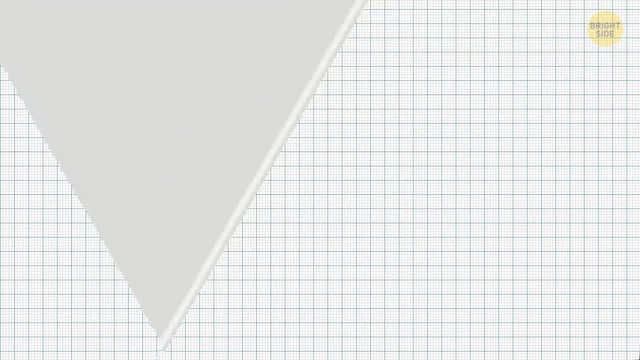 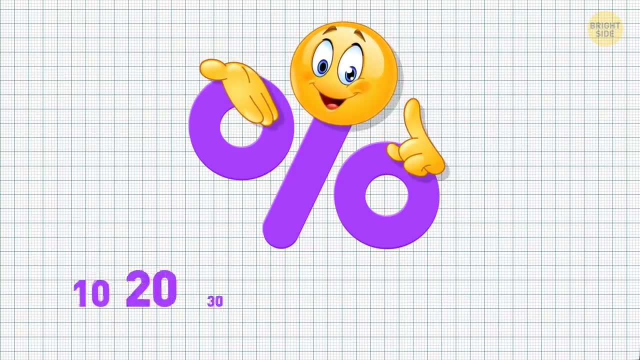 Which results in 957.. If you know the multiplication table well enough, finding out percentages will be a piece of cake. The only downside of the following method is that it can only be used with round percentages of round numbers. But hey, that's already something. So if 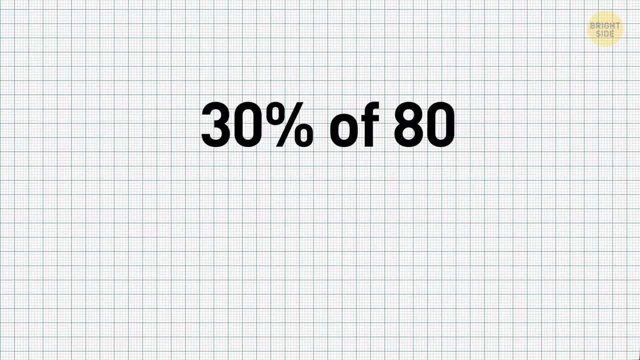 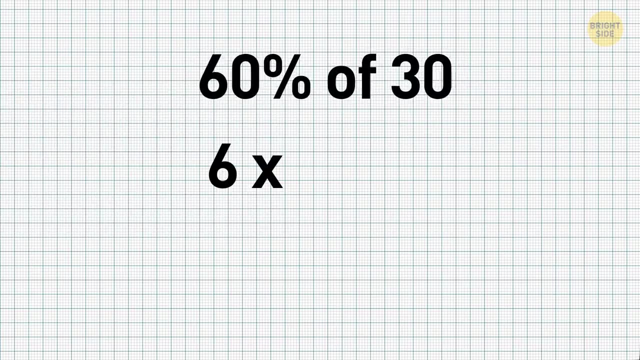 you want to find out 30% of 80,, you just need to ditch the zeros and multiply the tens places of these two numbers. 3 multiplied by 8 will be 24.. Same can be done with any rounded percentages and numbers. 60% of 30 will be 6 multiplied. 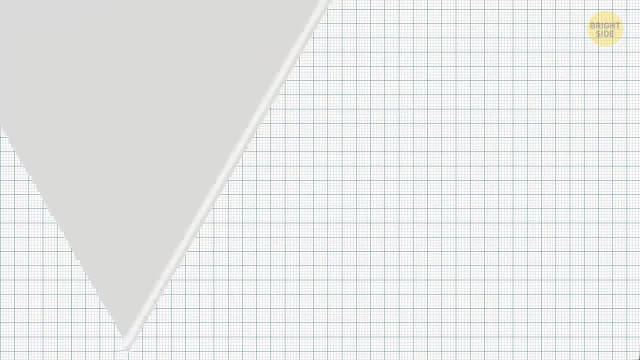 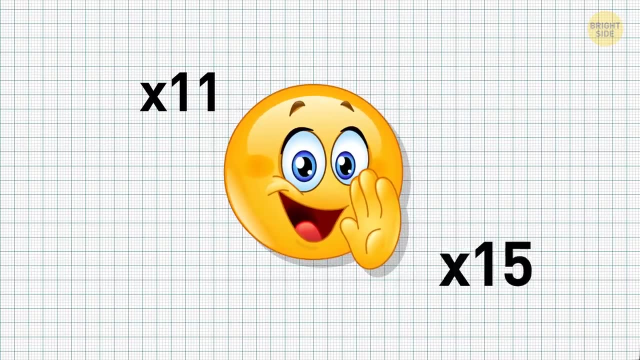 by 3, equaling 18.. Now let's get back to simple multiplication again. We've covered multiplying by 11, but what about 15?? Let's try it with multiplying 64 by 15.. First, add a zero to the first number. 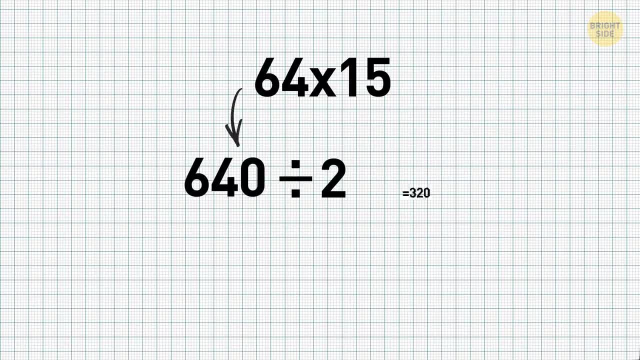 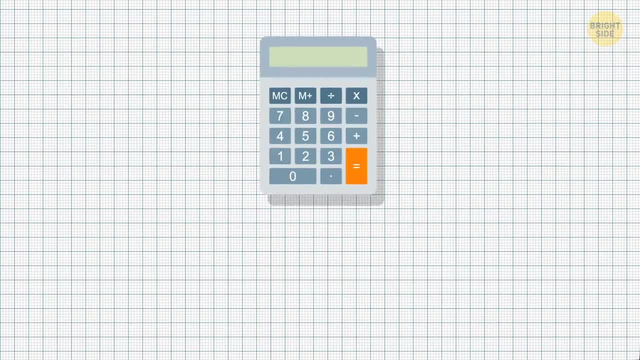 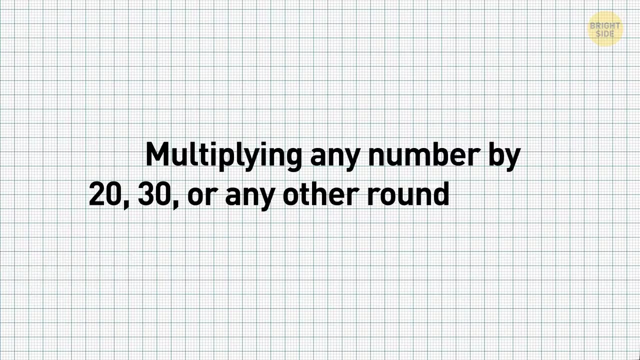 it using the calculator, but the principle is easy to grasp. You first multiply your number by 10, then multiply it by 5, which is half of 10.. Get it And add those numbers. A similar method applies to multiplying any number by 20,, 30, or any other round number. 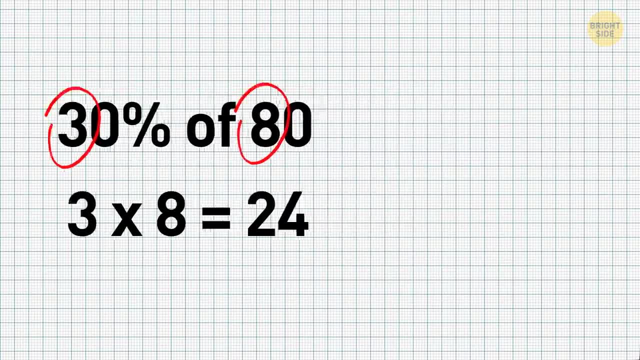 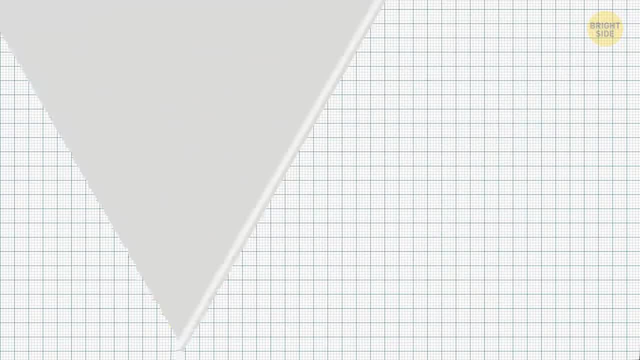 Same can be done with any rounded percentages and numbers. 60% of 30 will be 6 multiplied by 3, equaling 18.. Now let's get back to simple multiplication. again, We've covered multiplying by 11,, but what about 15?? 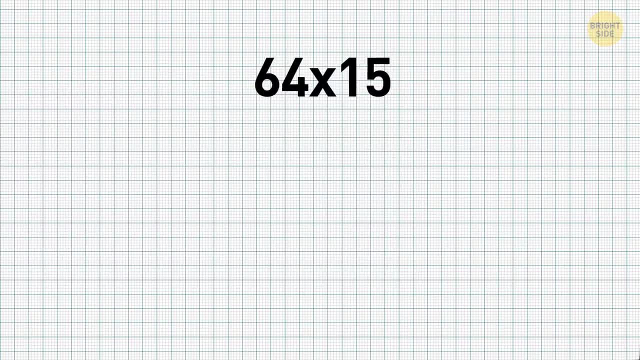 Let's try it with multiplying 64 by 15.. First add a zero to the first number, making it 640.. Now divide it by 2. Resulting in 320.. And next add the two numbers you've got. 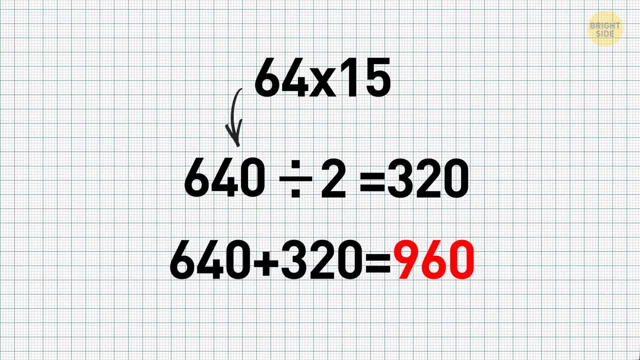 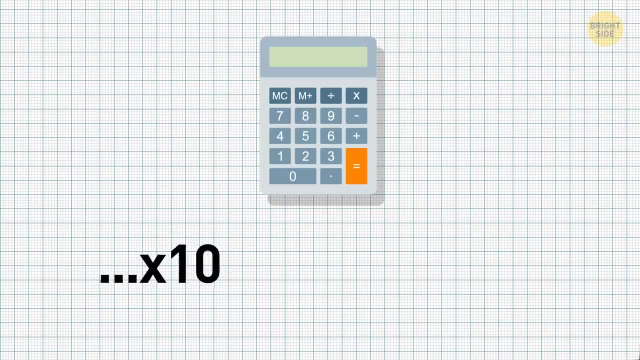 640 plus 320 equals 960.. You can verify it using the calculator, but the principle is easy to grasp: You first multiply your number by 10, then multiply it by 5, which is half of 10.. Get it. 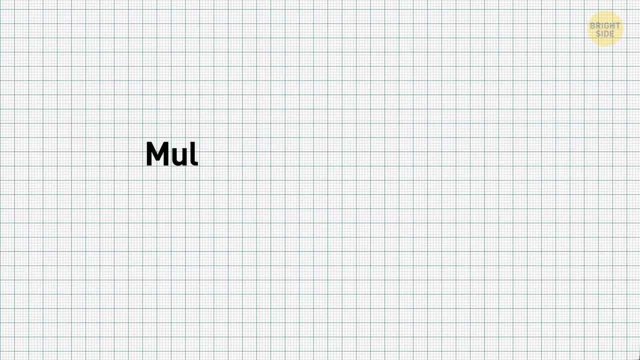 And add those numbers. A similar method applies to multiplying any number by 20,, 30, or any other round number. Let's say you want to multiply 41 by 30.. First add a zero to your number, making it 410. 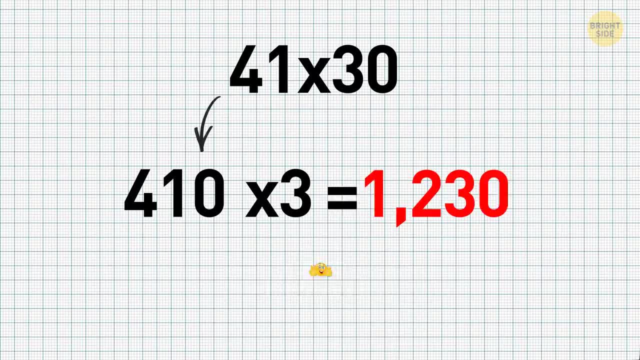 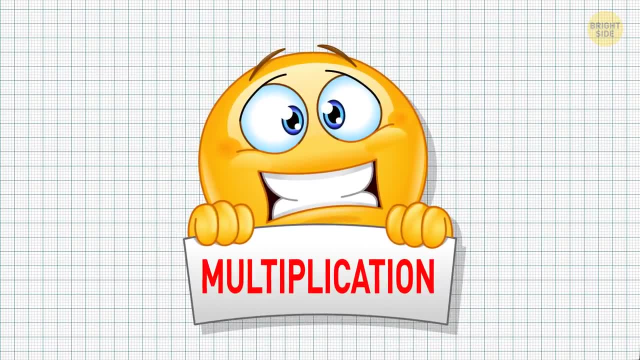 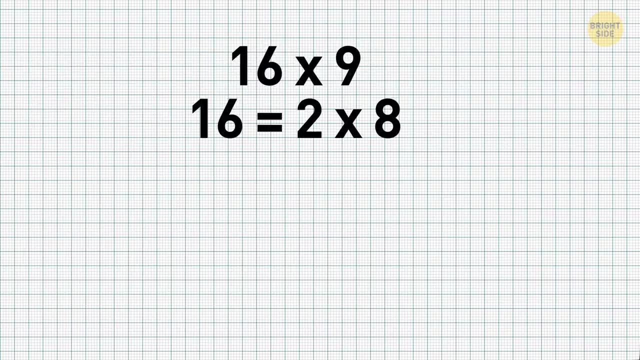 Now multiply it by 3, and you'll get 1230.. In fact, multiplication basically boils down to a number of additions performed in a row. Let's try multiplying 16 by 9.. 16 is 2 times 8,, which converts our task into 2 times 8 times 9.. 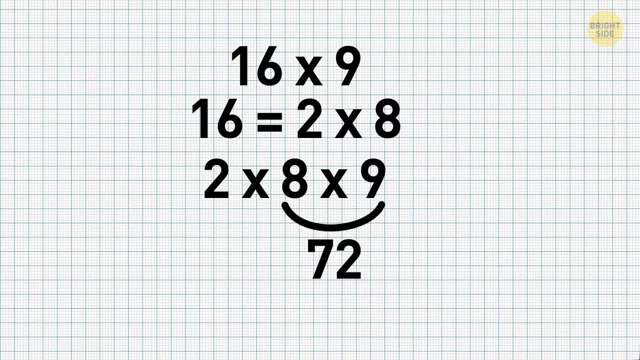 Since it's a number, we can multiply it by 9.. Since 8 times 9 will be 72,, we just need to add 72 with another 72, which gives us 144.. Let's take it up a notch and multiply two-digit numbers between each other. 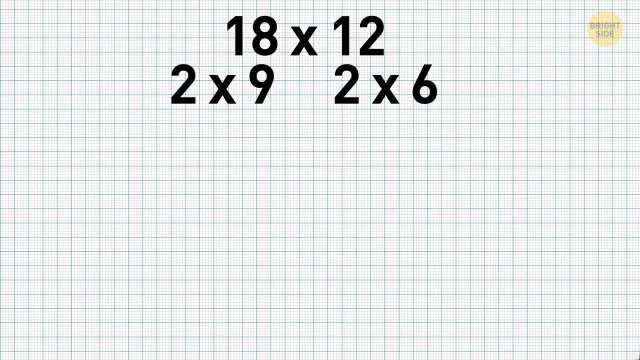 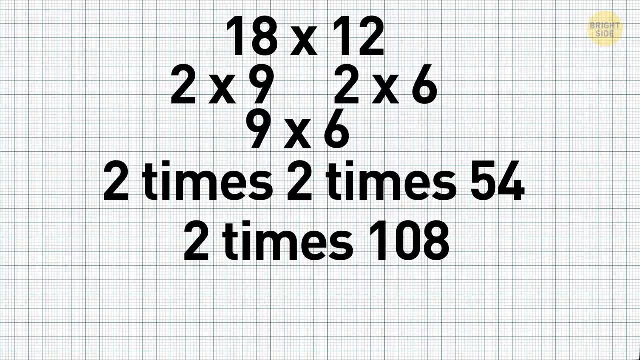 Say 18 times 12.. We can unfold these two numbers as 2 times 9 and 2 times 6.. Next multiply 9 and 6, resulting in 2 times 2 times 54. One step further, One step further, and we get 2 times 108, which leaves us with 216. 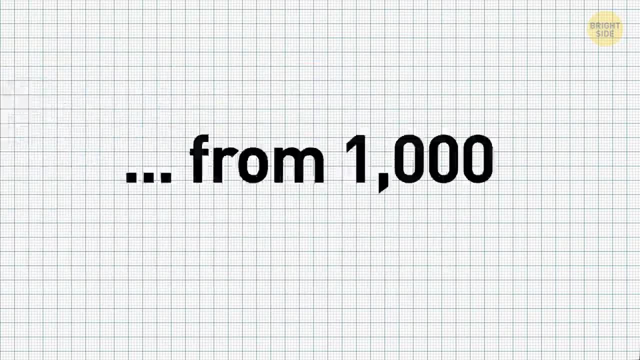 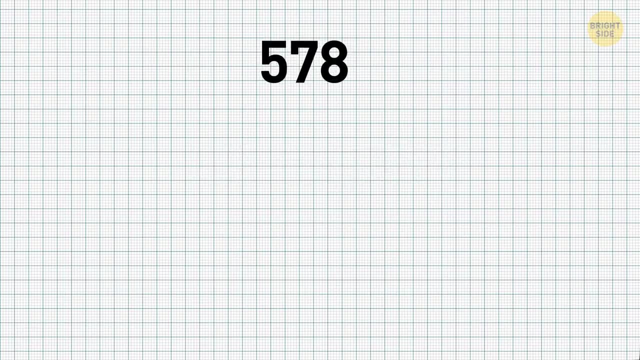 Subtracting can also be a headache with large numbers, But there's a simple trick to subtract any three-digit number from 1,000.. Let's take 578 as an example. What you need to do is subtract the first digit from 9.. 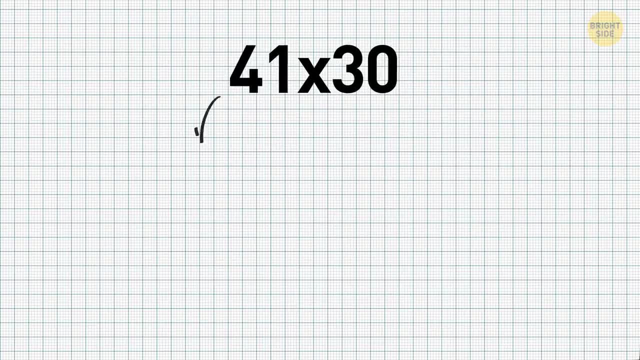 Let's say you want to multiply 41 by 960.. That's the answer. Now let's multiply 41 by 30. First add a zero to your number, making it 410.. Now multiply it by 3, and you'll get 1230.. 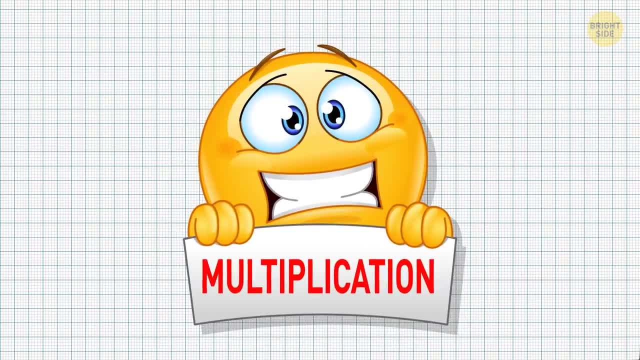 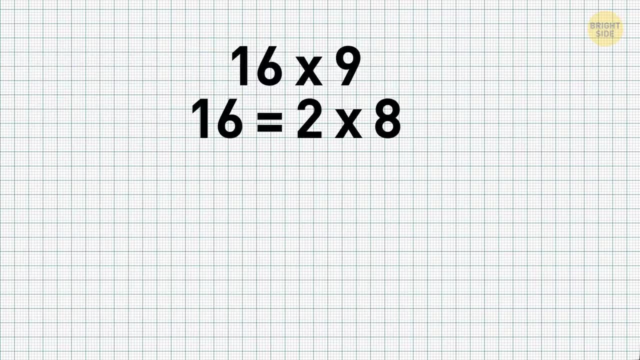 In fact, multiplication basically boils down to a number of additions performed in a row. Let's try multiplying 16 by 9.. 16 is 2 x 8,, which converts our task into 2 x 8 x 9,, since. 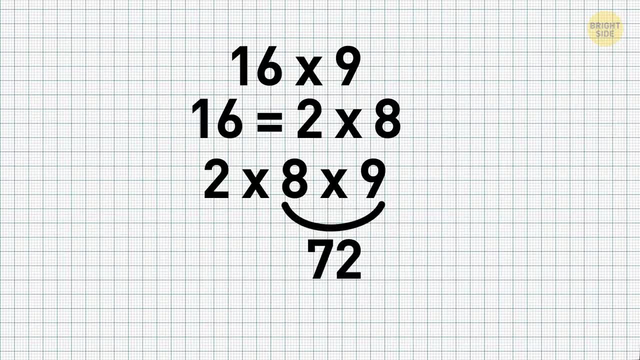 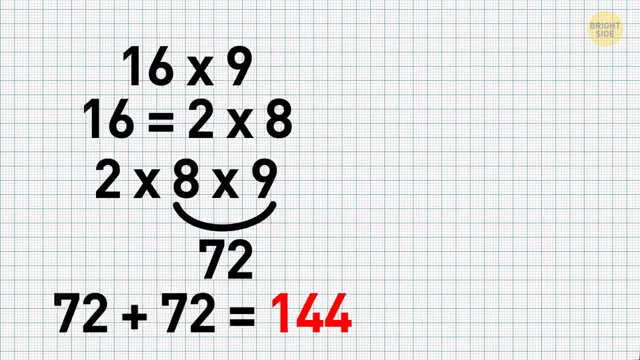 8 x 9 will be 9.. 9 will be 72.. We just need to add 72 with another 72, which gives us 144.. Let's take it up a notch and multiply two-digit numbers between each other. 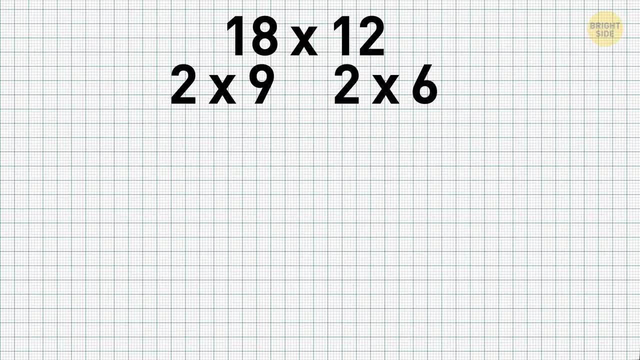 say 18 times 12. We can unfold these two numbers as 2 times 9 and 2 times 6.. Next multiply 9 and 6, resulting in 2 times 2 times 54. One step further and we get 2 times 108,. 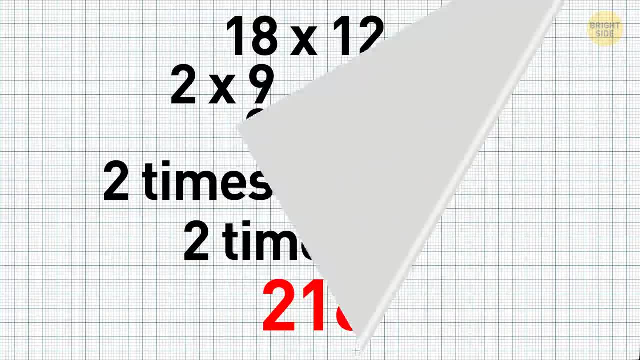 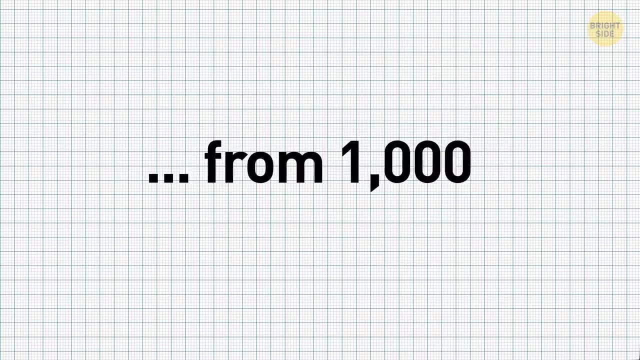 which leaves us with 216.. Subtracting can also be a headache with large numbers, but there's a simple trick to subtract any three-digit number from 1,000.. Let's take 578 as an example. What you need to do is subtract the first digit from 9.. 9 minus 5 equals 4.. 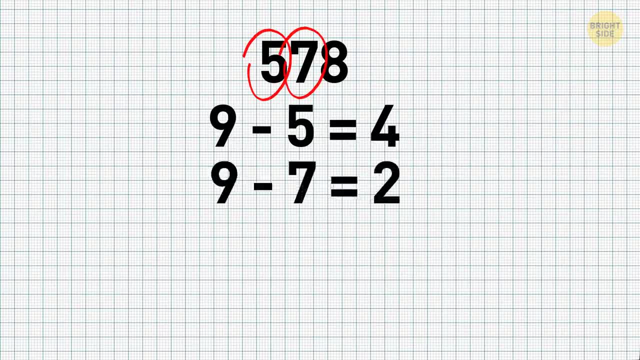 9 minus 5 equals 4.. Let's take 578 as an example. What you need to do is subtract the first digit from 9 as well: 9 minus 7 is 2.. And finally, subtract the third digit from 10.. 10 minus 8. 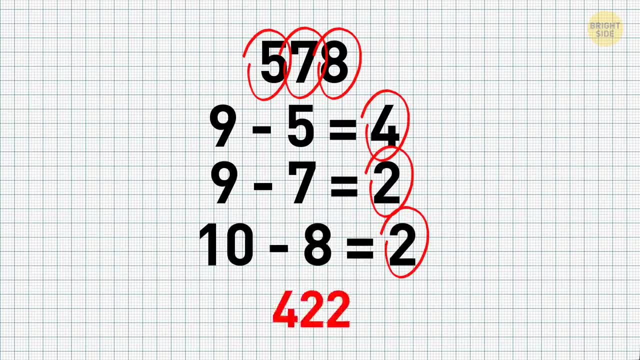 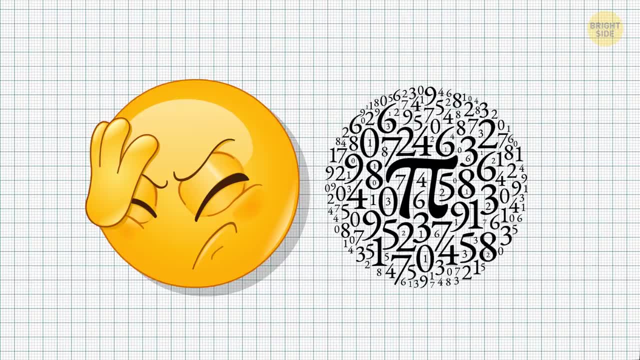 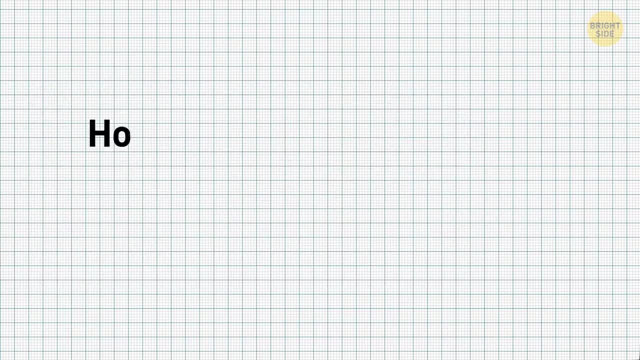 gets you 2.. Now place your results together. 422 is your answer. The number of pi is infinite and the digits after the point go in a seemingly random order, but there's a simple technique to memorize. the first six of them Say the phrase: how I wish I could calculate. 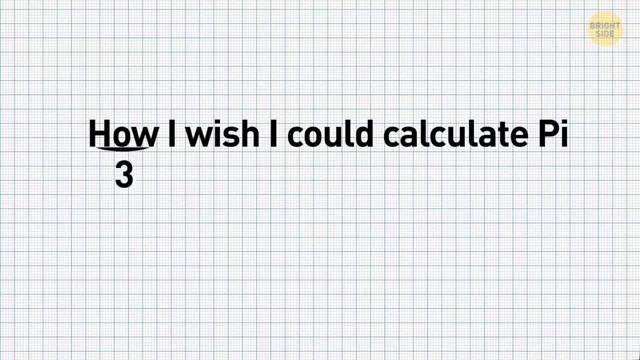 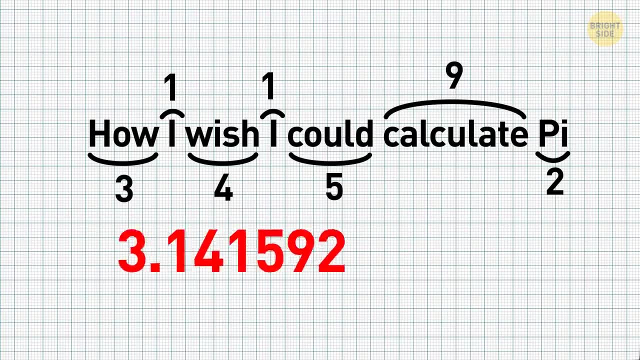 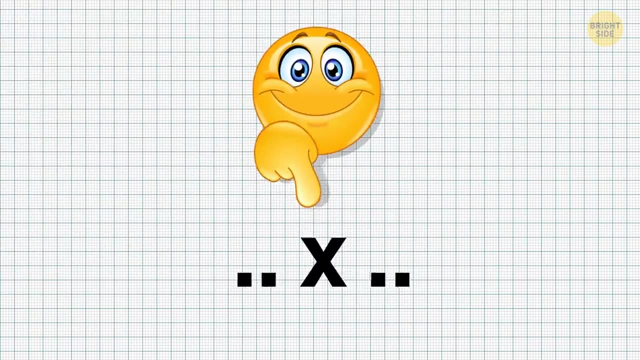 pi out loud or write it down. Now count the letters in each of the words and you'll get the three and the first six digits after the decimal 3.141592.. You can multiply large numbers between each other in your head easily, but take note that this trick only works with numbers in.